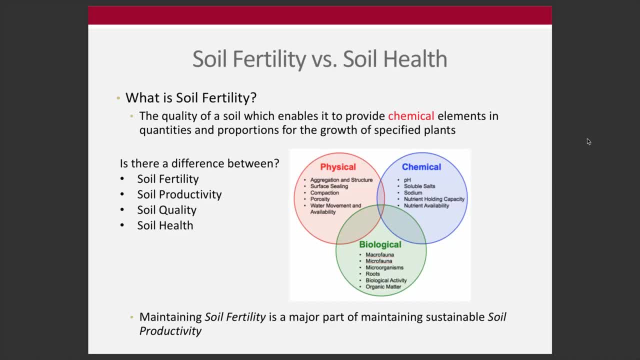 So soil fertility, again the topic of this entire course we can think about or at least traditionally define, the Havlin textbook talks about- I think this is the definition- but the quality of soil which enables it to provide chemistry. So fertility in many ways has historically been associated with soil chemistry and the ability of that soil to essentially provide the important chemical nutrients over growth. 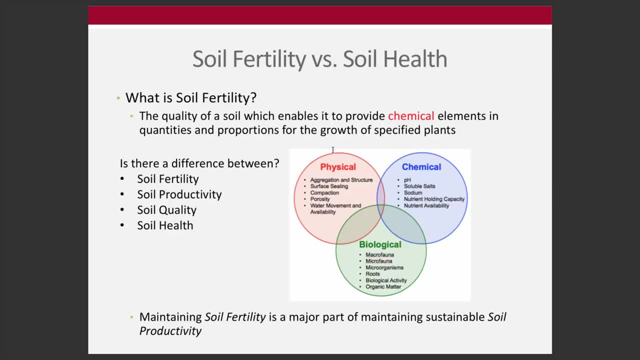 And you know, you've likely all seen something like this picture before- where we've got soil that's made up of a physical, chemical and a biological. And if you look at the chemical components, for example in soil there's a chemical component, a biological component. 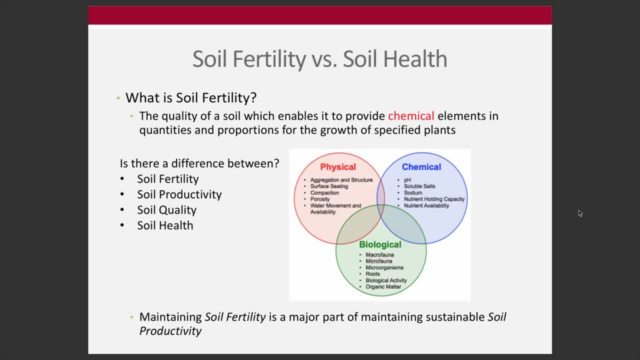 Those three things conceptually are distinct, but the reality of how they come together in this integrated matrix of a soil, clearly there's a very intimate integration of the physical piece with the chemical piece and with the biological piece And each one of these play off each other and there's feedbacks between one and the other, etc. etc. 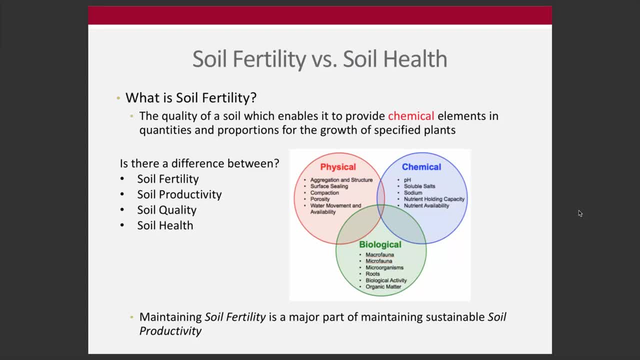 So fertility, thinking about chemistry, But what's the difference between fertility and soil health? fertility and productivity, soil quality, even soil health. So is there a difference? I would say yes, there likely are differences between those terms and we should understand some of these differences. 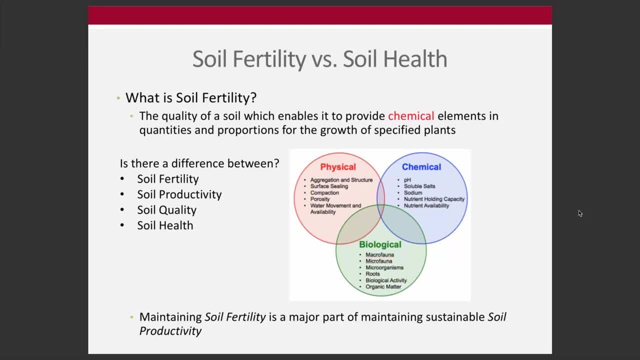 I will say that also, that particularly as it's practiced and particularly in agriculture, language is very imprecise and used. you know there's a lot of terms that are thrown around, And so I would say soil productivity within that umbrella. you know that's a crop or a plant focused. 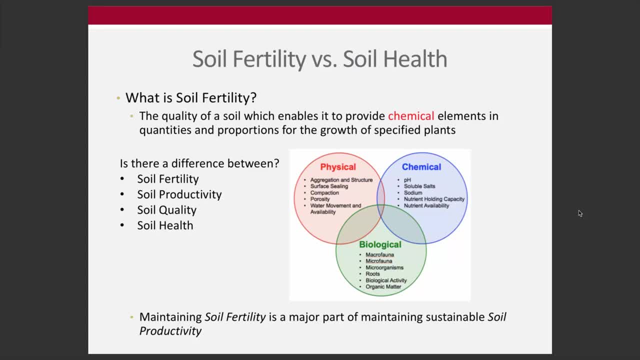 perspective. but fertility is a piece of kind of soil health. So soil health might be a little bit more encompassing and fertility is a major part of maintaining productivity. okay, So again, are we managing? you know, a lot of times soils have 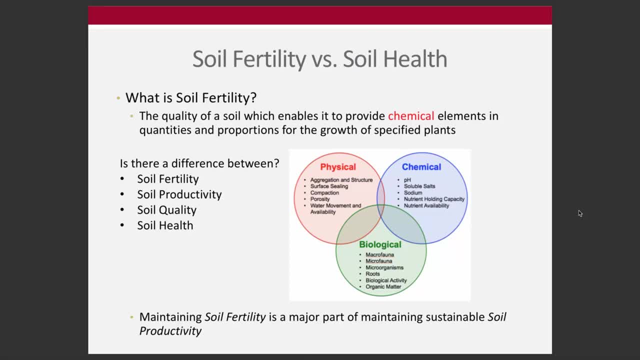 inherent value in their own right, But so many times we are interested in studying soils and thinking about soils in the context of you know the utility and the value that they provide for us, And a major part of that, of course, is the ability for them. 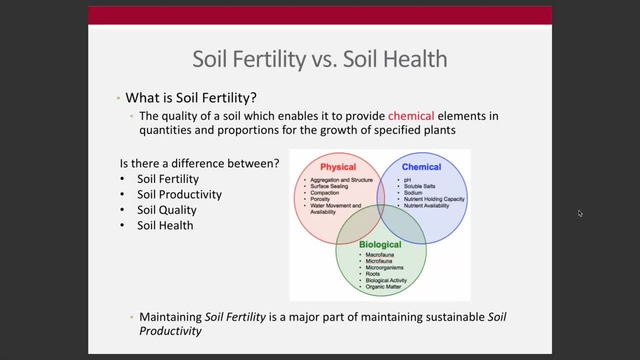 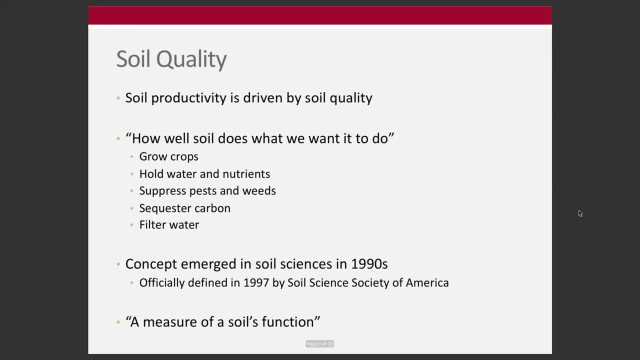 to produce, you know, healthy and productive plants And in an agricultural context it would be crops and harvestable product from crops, So soil quality. So you know, thinking about this idea again of like kind of like evaluation, evaluating or assigning value to what soil is. 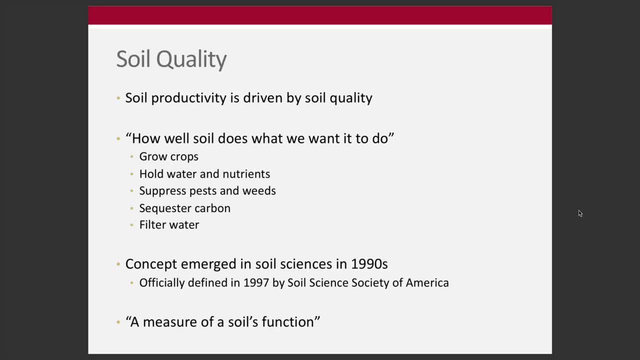 And so how well a soil does what we want it to do, And that's you know. there's again. this is kind of like a subjective take on this, because it's asking an individual to, you know, assess what they, what they think or what they believe. 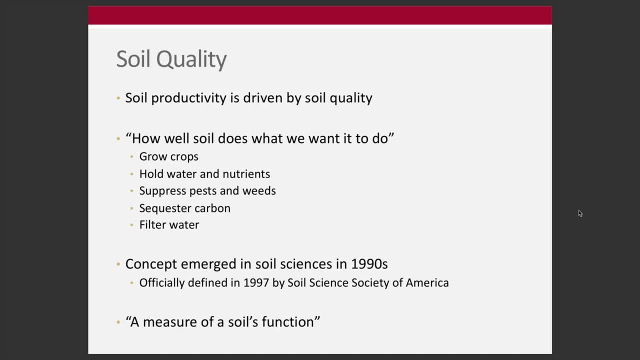 or what they value in terms of this output or this function. So we can talk about growing crops, We can talk about holding water nutrients, suppressing weeds, sequestering carbon, filtering water. you know all these things. Soil quality was really this original concept. 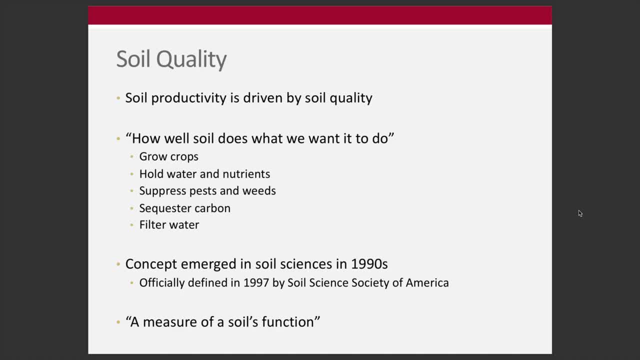 People had thought about this for many, many years before And But as kind of like a vetted scientific thing, right sanctioned by soil scientists. it was a concept that emerged in the 90s and there was a lot of talk and discussion of this. 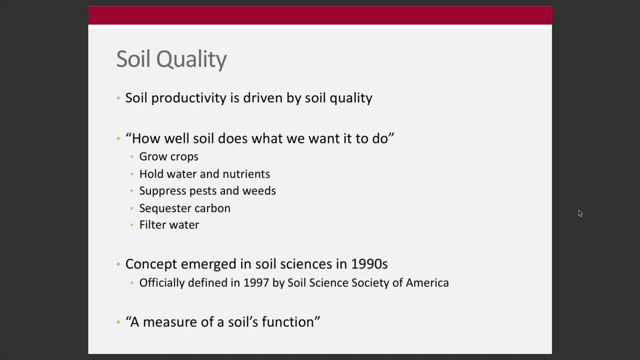 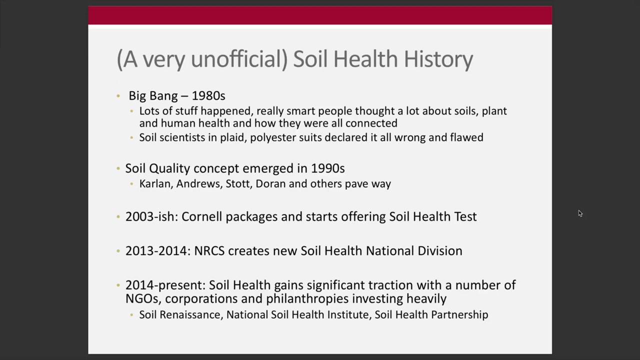 And then in 1997, the kind of governing soil science body, Soil Science Society of America, officially adopted this concept- and it's a really integral to that- as a measure of a soil's function. What's that soil do? Okay, So you know we can take a step back and think about soil health. 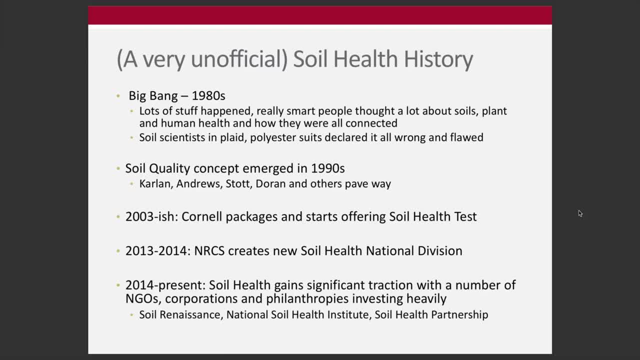 and soil quality. I view those two concepts as synonymous. Some people do, some people don't, But I don't think you know. we've already spent a little time about some of the semantics here. We can move on, but you know it's, this is a bit of a tongue. 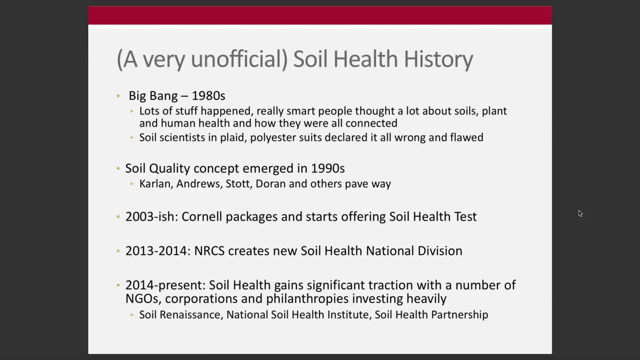 and cheek kind of slide here. but you know, from the Big Bang to the 1980s there's a lot of stuff happened. Really smart people thought a lot about soils, plants and human health. You know, a healthy soil makes a healthy plant. 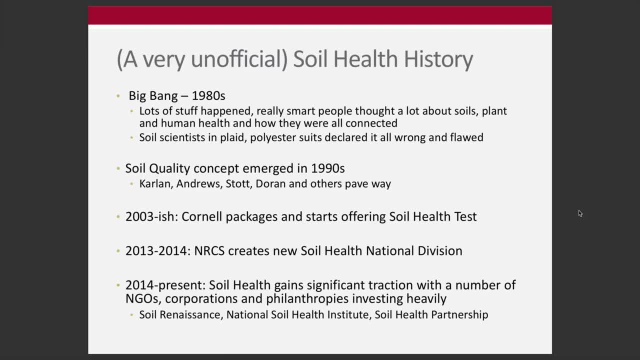 makes a healthy human, et cetera, et cetera. How the interconnectedness of all this. Science is very good at some things- Reductionism is, you know, a primary trait of science. But what science is really bad at is evaluating. 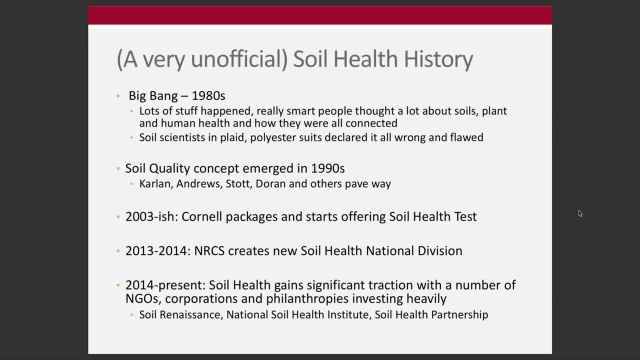 and identifying really complicated networks and interactions. right, And that is in a nutshell what soil health or soil science is, And this idea of going from a complex soil to a complex community of plants and then to the complexity of human and human biology, or animal biology, it's you know. 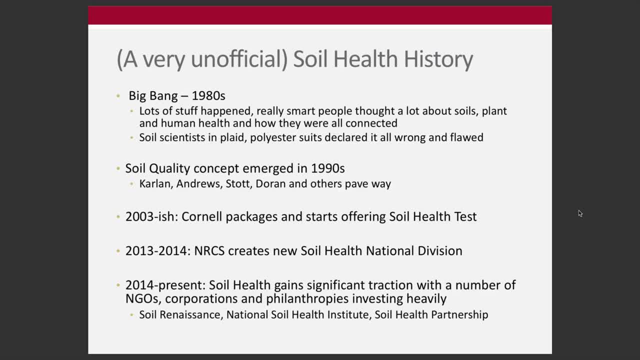 that's very, very difficult to demonstrate scientifically. Soil scientists- in plaid suits, you know, said: oh, that's all hogwash. We've got to. you know, when we're talking about science, it's got to be reductionistic and it's got to be, you know. 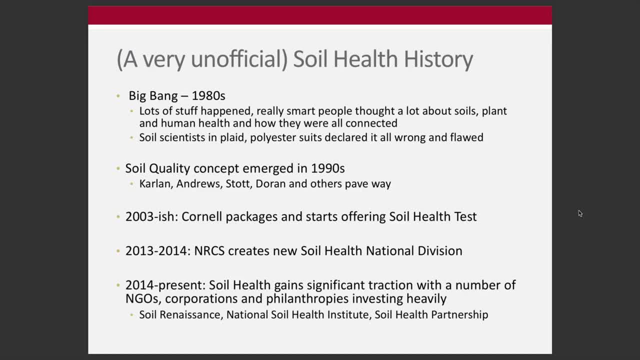 things that we can quantify and things that we can measure. So this idea of health or quality encompasses, you know, this concept that soils are more than just the sum of their parts, It's more than just the number of parts, It's more than just you know how much biological, microbial, 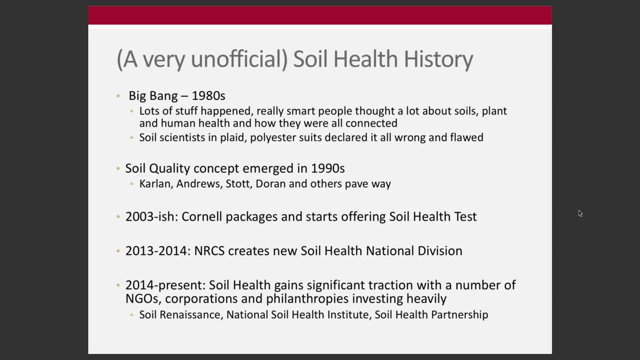 biomass there is how much. you know what's the bulk density value. All these things can come together to make more than just the sum of those things, okay. So again, the soil quality concept emerged in the 90s. 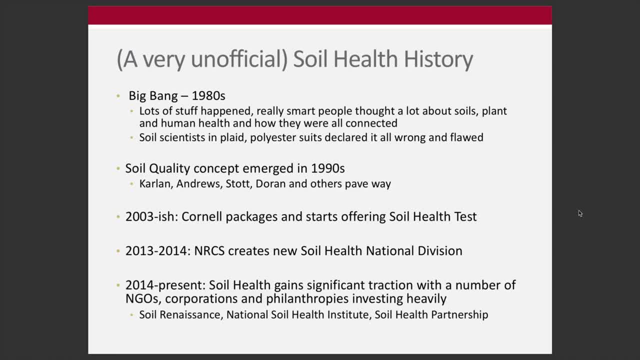 2003 was really kind of in my mind where a lot of things really started to happen in. Cornell Officially started offering their soil health tests, okay, And so Cornell has been a leader in this field for a long time. They broke from this concept of soil quality very purposefully. 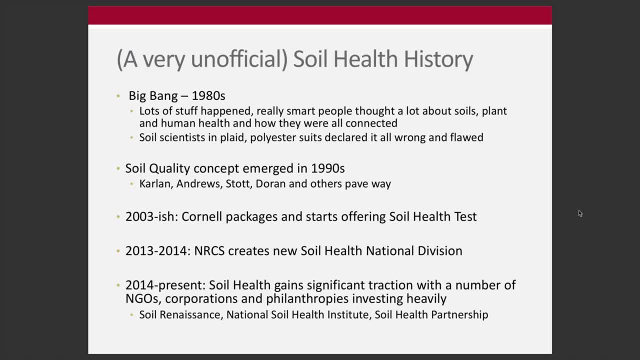 and they'll talk about why this concept of health is just more intuitive, right, So we can talk about quality. that makes sense. People understand intuitively quality, But health of a soil and the health of a person, you know it's very intuitive. 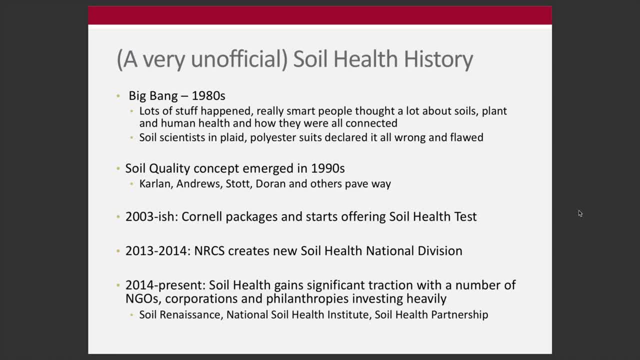 That you can understand that we can measure your blood pressure, We can measure, take your temperature, We can measure a number of things, And those all might be fine, but you still might not be feeling quite well in any given day. And you know, this is again this kind. 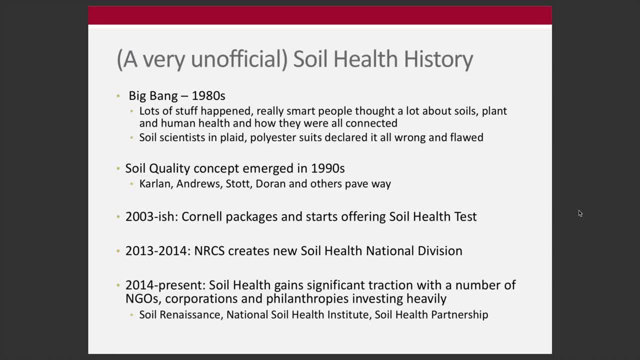 of inherent concept of health And so anyways. so Cornell has been offering this soil health test for a number, you know, for 15 years-ish, And then in 2013-14, the National Resource Conservation Service, NRCS. this is a branch of USDA. 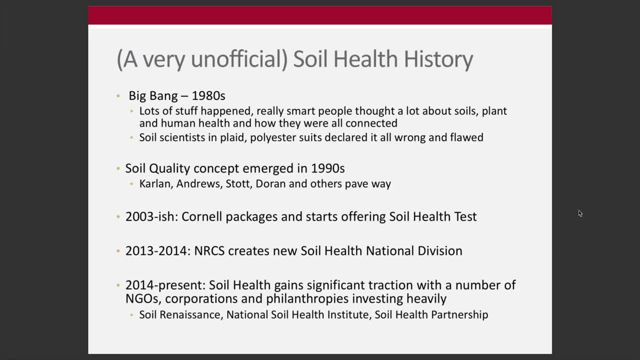 if you're not familiar with them. They are really charged with soil conservation and water conservation And they do quite a bit of work. nationally They created a Soil Health National Division, So NRCS has had historically the last 20-30 years. 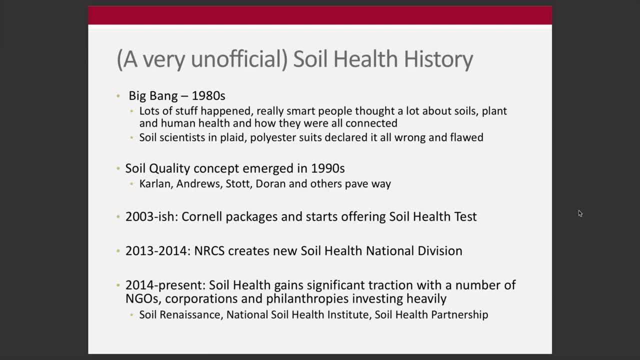 been mapping a lot of soils. So if you, you know, you go. we have a national database, the Soil Survey, where all soils in the United States- not all of them, yet they're still, you know, doing some soils. 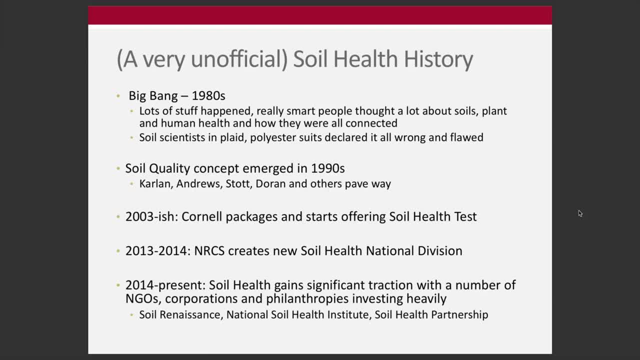 still mapping soils in remote areas, But there's been a tremendous investment by the federal government in mapping and essentially like taking an inventory of the soil, All the resources that we have. So if you, you've likely encountered this at some point, like you know. 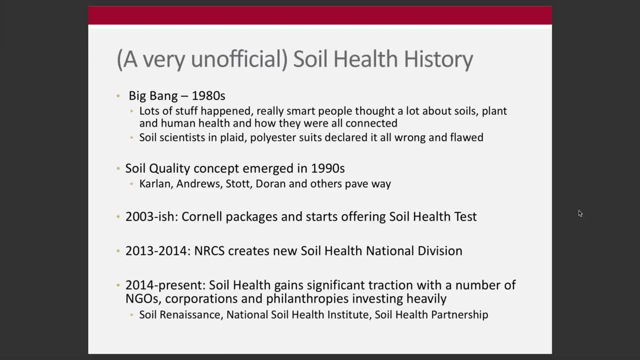 the Soil Survey. it's called the SERGO, But this is the work that they did. They do a bunch of conservation work, work with growers for, you know, incentivized payments for growing cover crops, or working with like Conservation Reserve Program. 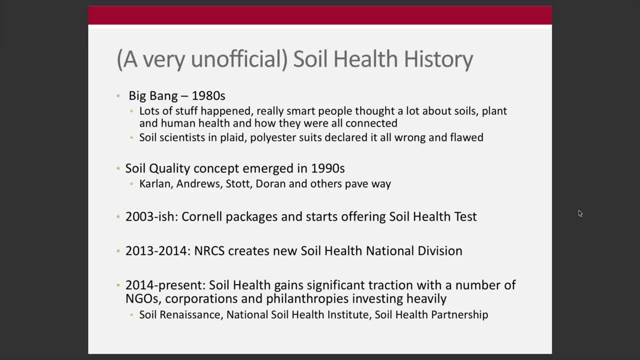 or EQIP, where you're setting aside very sensitive, highly erodible soils out of production or implementing riparian buffer or doing all kinds of things that improve soil and water quality. okay, So that's their charge, But they said that this is a thing that we feel very strongly. 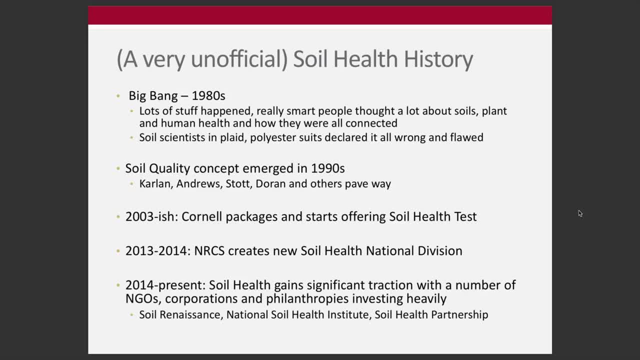 that we want to invest in and has lasting potential for conservation purposes, And so they essentially created a sister division to their Soil Resources Soil Mapping Division. So it was a big move and a big- you know, major- statement from a large federal agency about soil health and why. 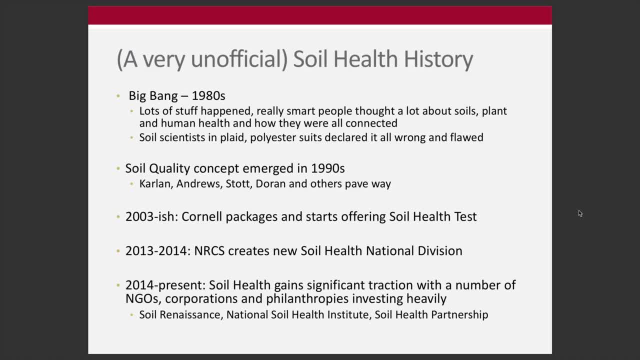 we think it's very important And it's a good framework for conservation. okay, So it's really. I mean, it's not been very long folks, It's been. you know, really since 2014- that a lot of this has kind of blown up. 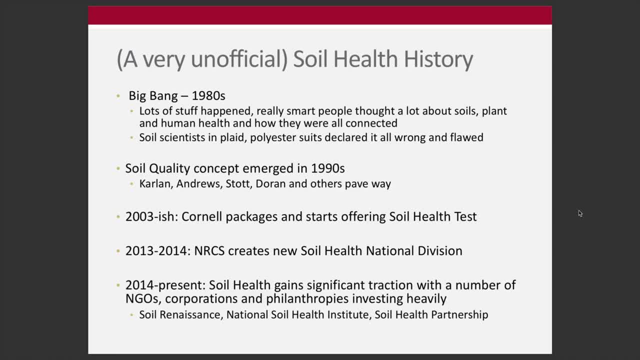 There's been a lot of input from corporations, you know, like the Walmarts, the GMs, the Monsantos of the world that have decided to, you know, to do this work. They've decided, prioritized that this is something. 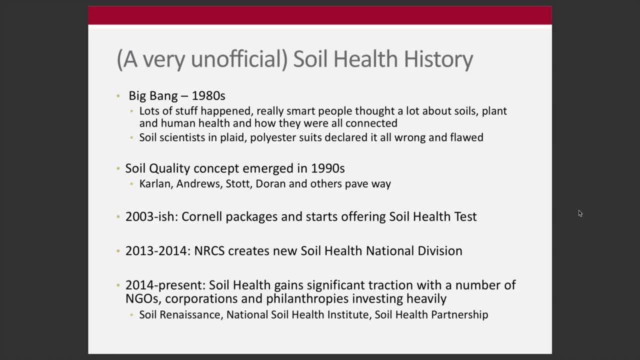 that they want to invest in. So you know we could get into all this. We don't really have time. but, like the Soil Renaissance, there's a National Soil Health Institute that's formed in the last several years. There's a Soil Health Partnership, which is a large 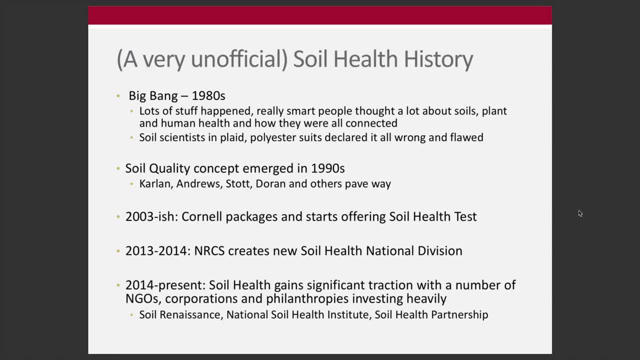 again mostly corporate-driven initiative dealing with soil health and soil health-promoting practices. So it's very hard to pick up a trade magazine or even like a scientific journal And not see the word soil health. So it's clearly, you know, you could argue if it's a buzzword. 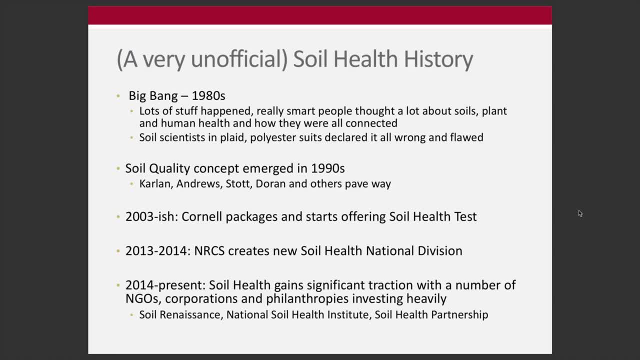 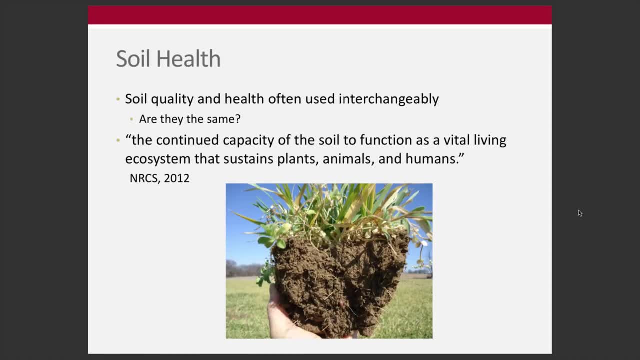 if it's here to stay, if it has the you know sustaining power. but suffice it to say there's a lot going on right now. So, health and quality: are they used the same? Are they the same? I will use them the same. 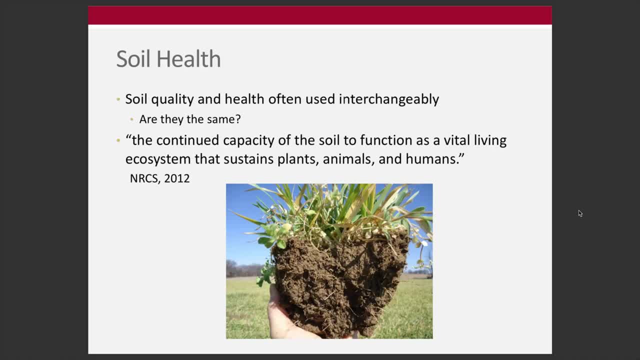 We can have a conversation about. you know differences, But NRCS has defined this as the continued capacity of the soil to function as a vital living ecosystem that sustains plants, animals and humans. right, So that's what kind of technically the definition. 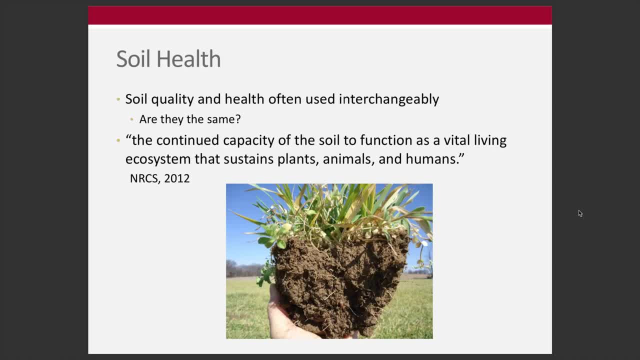 of soil health is, but that's not particularly helpful if you actually think you know it's so broad, right? And it's one of these issues with soil health is that people think of it very differently, all right. So again, this idea that everyone's you know. 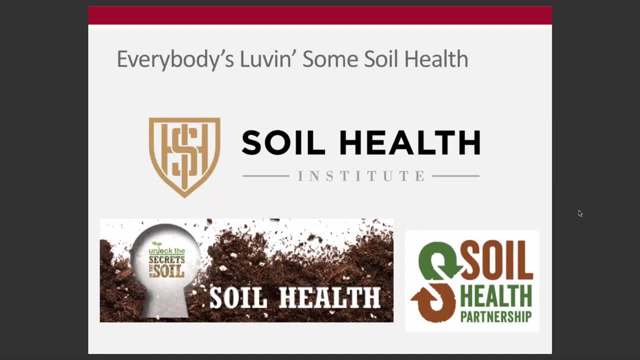 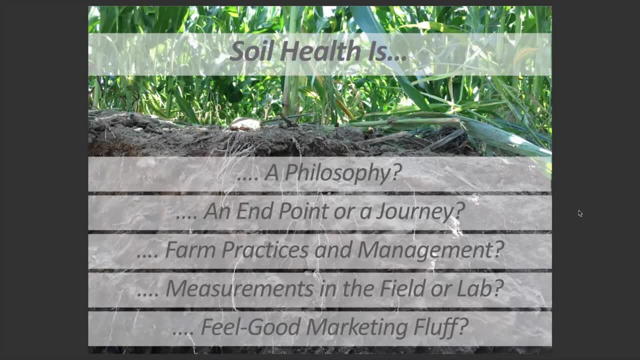 really into soil health right now, and there's a lot of different examples that we could, we could talk about, but we'll move on for the sake of time, right? So soil health: what is it right? Is it a philosophy? 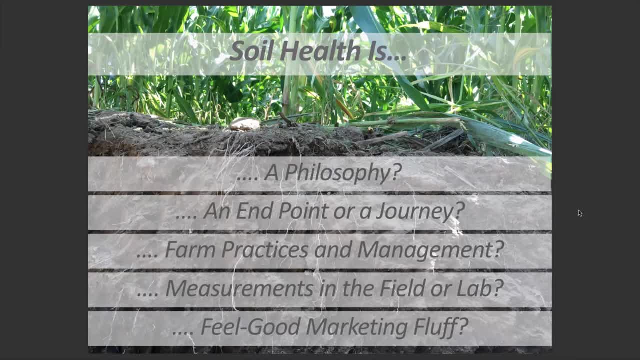 Is it an endpoint or is it a journey? Is it mostly about farm practices and management, you know, just conservation practices? Is it mostly about quantifying soil, about taking measurements in the field or in the lab, right, Or is it just all too squishy and too squiggly that it's 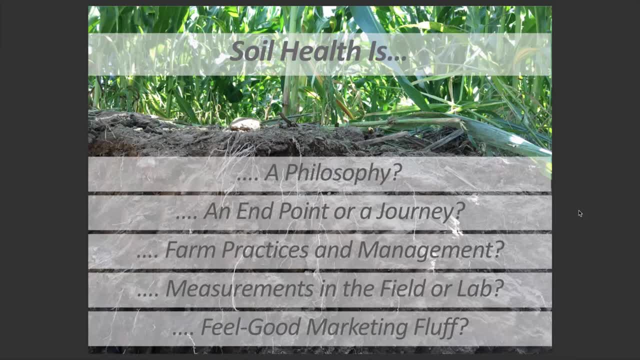 it's hard to quantify, it's hard to define, it's just this feel-good marketing fluff, right? So maybe a little bit of all this, maybe not. I mean this, it really depends. These are open-ended questions. 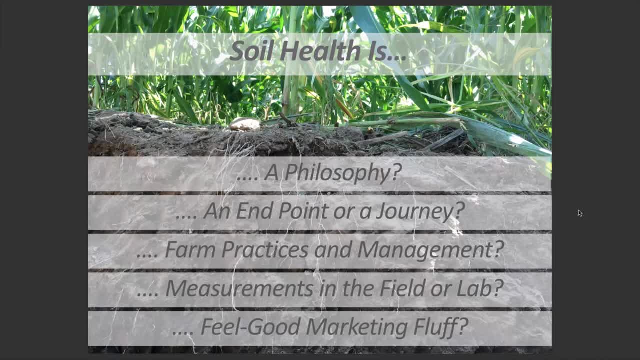 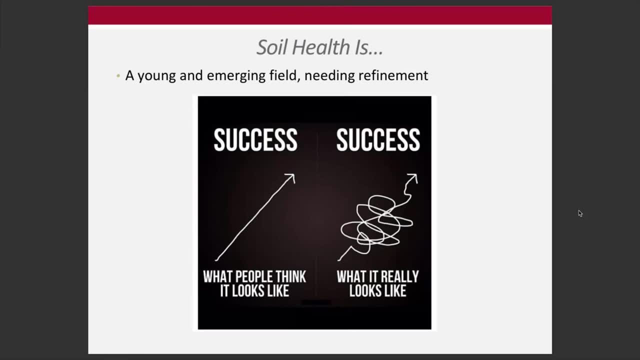 It depends on who you ask You're going to get. you ask 10 different people, you'll likely get 10 different answers about each one of these, right? So you'll have to pardon my kind of cheesy clip art here. 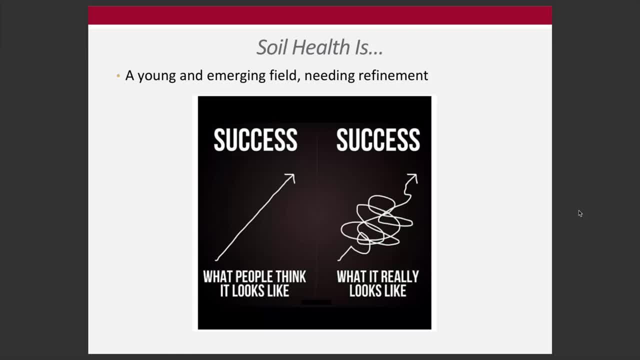 but soil health. I think it's important for us to understand it's a young and emerging field, right? It needs refinement. So it's not like we're just marching down this linear path and that there's going to be missteps and blah, blah, blah. 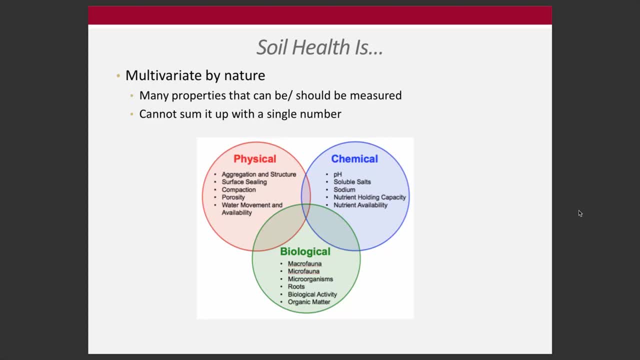 We also need to understand that soil health is multivariate by nature. What do I mean by that? Well, I mean you can't just look at one indicator at a time or one measurement at a time. We can't just look at pH. 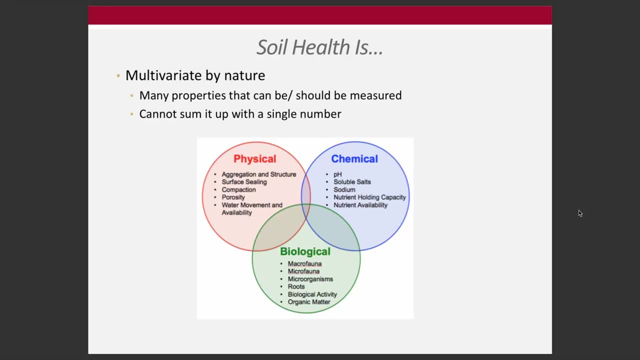 We can't just look at, you know, biological activity. We've got to look at all of these things collectively and kind of hold them, you know, upload them into our brain and hold them there and understand that there's a lot of relationships. 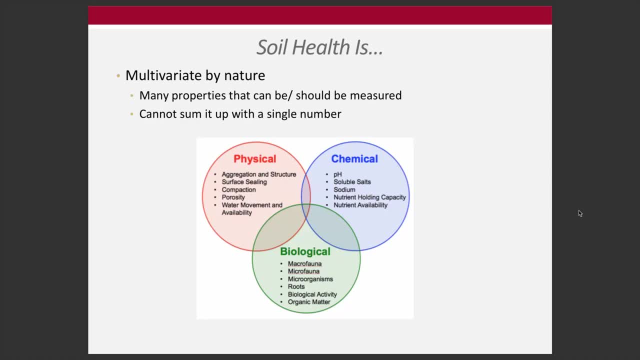 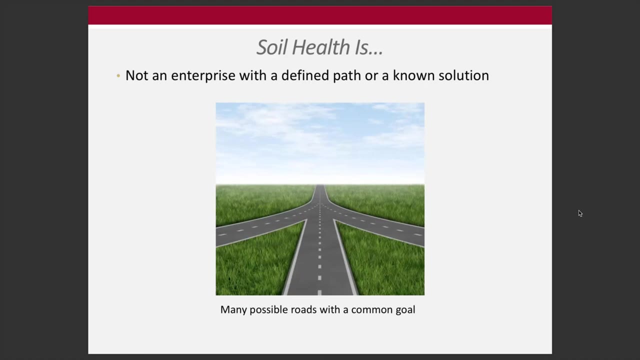 and a lot of interactions that occur, So we can't just sum all this stuff up into a single number, but there's many properties that make up this quality or this concept of soil health. So, and again it's like this bit of uncertainty. 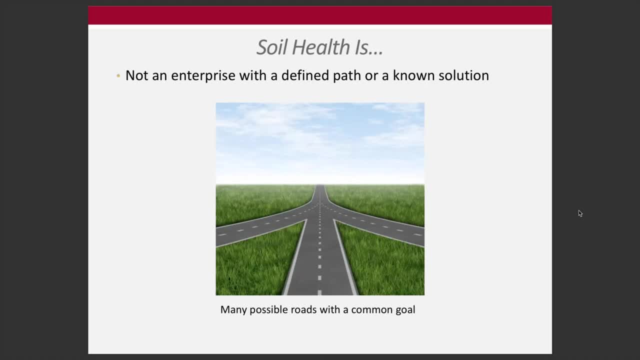 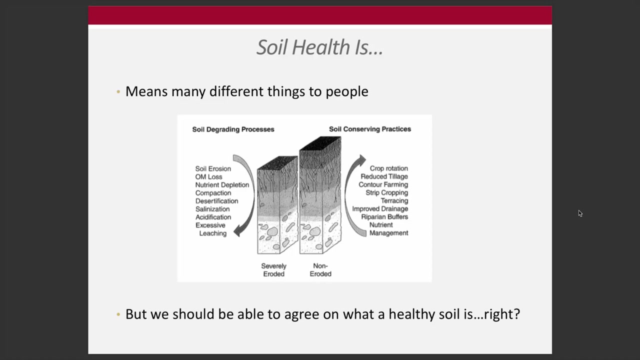 in terms of we don't know exactly where we're going, but you know there's a number of people trying to sort this stuff out in terms of where this field is going. So soil health means many things to different people. okay, 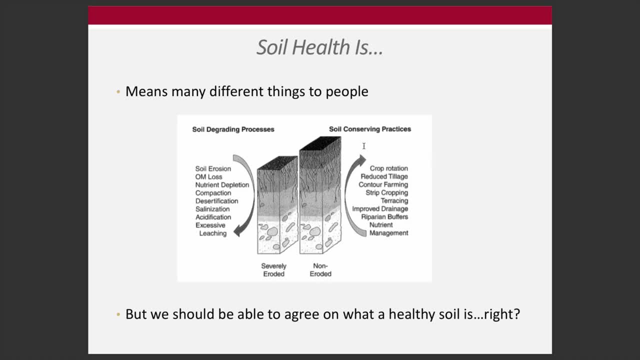 And you know, again, broadly, we can think about soil degrading processes like erosion, organic matter loss, nutrient depletion, et cetera, et cetera. We can think about, you know, soil conserving practices or processes. 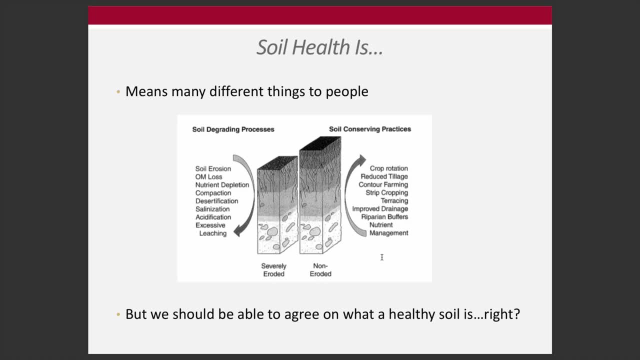 things we get with crop rotation, reduced tillage. you know best nutrient management, particularly for this class, right? So we can dichotomize: what's you know going to promote soil health, what's going to detract from soil health? 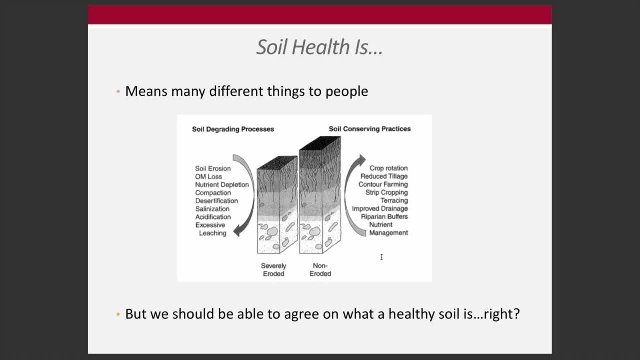 but we should all be able to agree on what a healthy soil is right. Even though there's like there's a lot of uncertainty or a lot of like lack of precision in the language that we're using here, we might be able to agree on what a healthy soil is okay. 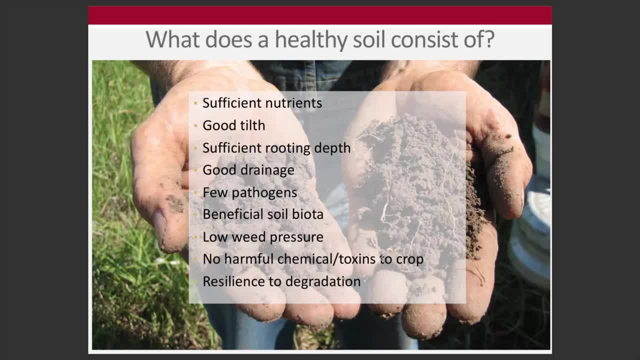 So I think most people- this is not going to be a list that is contentious, right Like we could debate some of these finer points, but for the most part people would understand that a healthy soil would have all these properties. 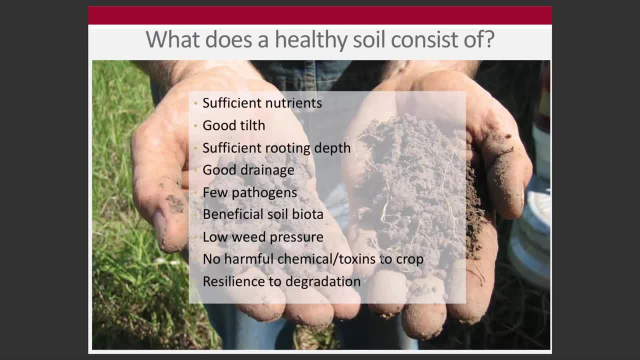 sufficient nutrients for plant growth, good till their structure. sufficient rooting depth so that those roots can really explore the soil and mine soil nutrients and water, et cetera, et cetera. Good drainage, so we don't have anoxic conditions occurring. 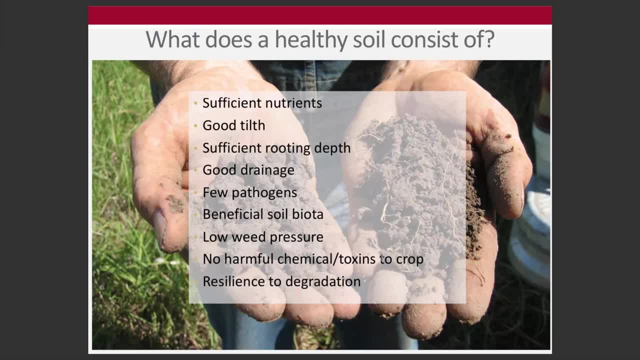 Low pathogen load with many beneficial soil microorganisms. Low weed pressure. you know, no harm for chemicals or toxins to crops, we don't you know. going into it. you know a super fun site might have really beautiful soil. 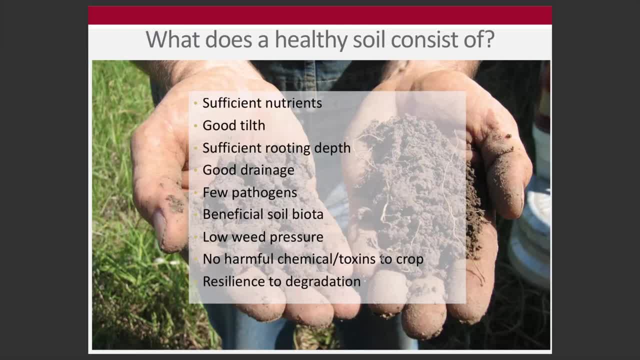 but if it's got some kind of pollutant, environmental contaminant, then most people would not call that a healthy soil And this idea of resilience to degradation right. So these are all things that you know we can kind of agree on in terms of what goes into soil. 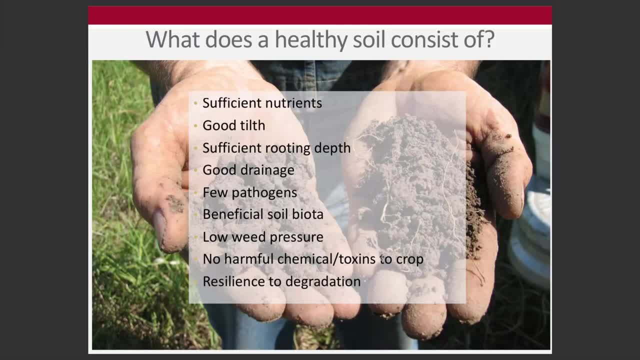 One of the challenges, though, is, if we look at this list, we look at sufficient nutrients. Well, what does that actually mean? What does sufficient nutrients mean? Or what does good drainage, or a few pathogens? We have to actually start measuring things right. 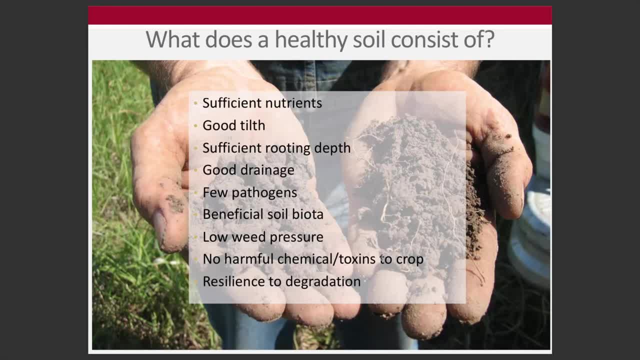 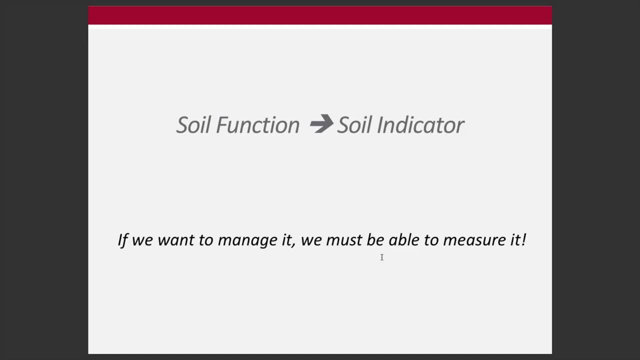 We have to start quantifying things, And the devil here is in the details in terms of how we actually quantify each one of these attributes or characteristics of a healthy soil. okay, So we'll get into that in a little bit. We need to move from soil function to an indicator. 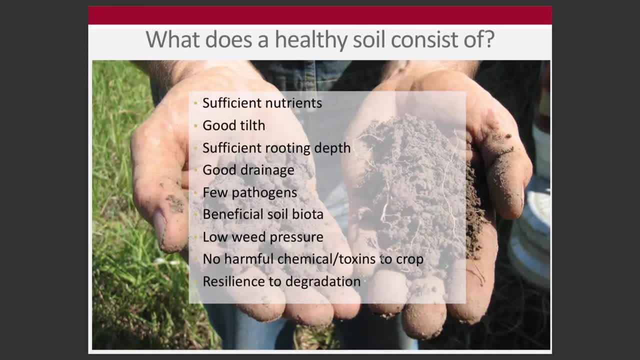 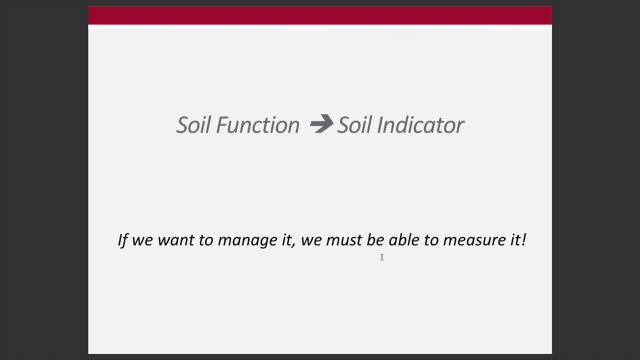 So I would say this last slide: these are all functions, right? So like good drainage, low weed pressure, dah dah dah, Those are functions of soil. But we actually need a measurement, We need an indicator to relate that. 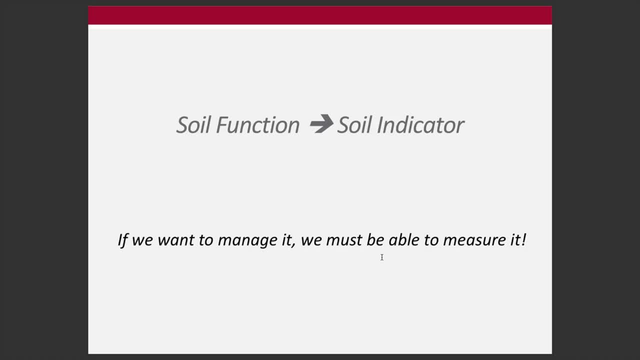 or reflect that soil function. So- and you know I say this all the time- but if we want people to manage a soil property, we must be able to measure it. You are never going to manage cholesterol if you never measure your cholesterol. 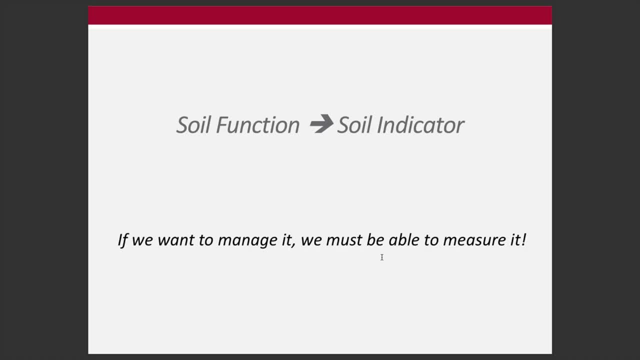 You're not going to be aware that you have high blood pressure if you never go get a checkup and get your blood pressure read right. So it's just like we can't be managing for soil properties that you know unless we are actually physically. 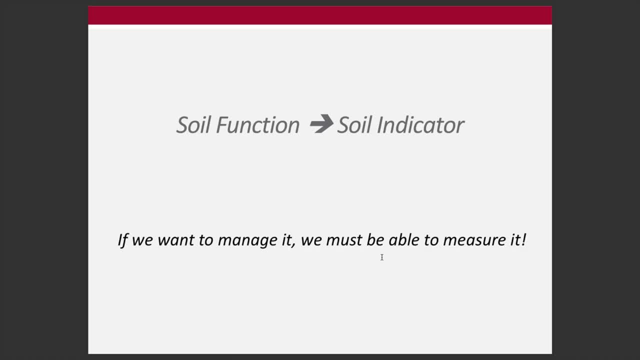 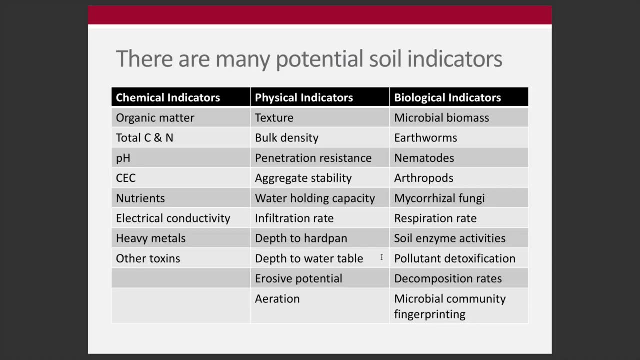 actively measuring them okay. So it's a really important thing to understand. Soil science has been around for a long time and we have lots and lots of measurements. We have lots of ways to actually quantify properties of soil. Those can broadly be defined into chemical indicators. 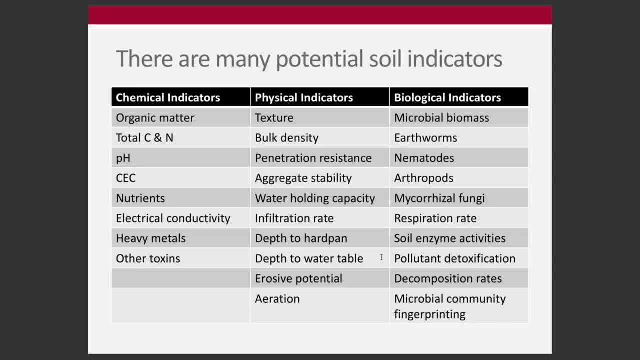 physical indicators, biological indicators. I'm using the word indicator and measurement synonymously here, So you know, let's not be confused about that. This is a table that lists, you know, different chemical, biological and physical indicators. In no way, shape or form, is this an exhaustive list. 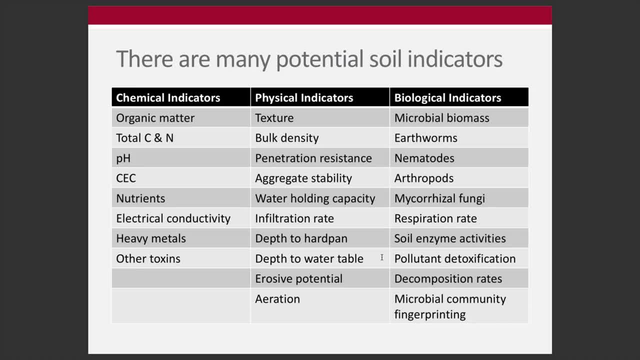 We've got you know entire textbooks that outline various, various manuals and provide standardized protocols to do that right, And so this is an important part of science, that this is what CEC is, This is how we measure it, And then you can reproduce CEC across many different labs. 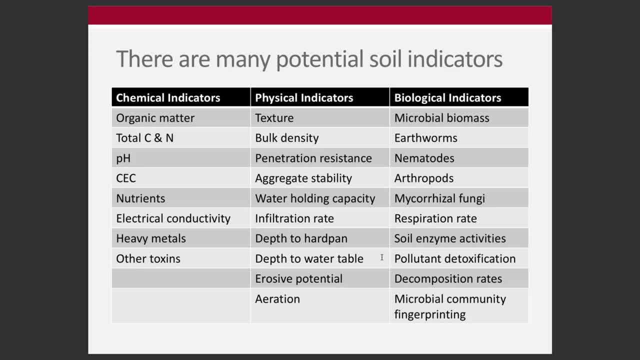 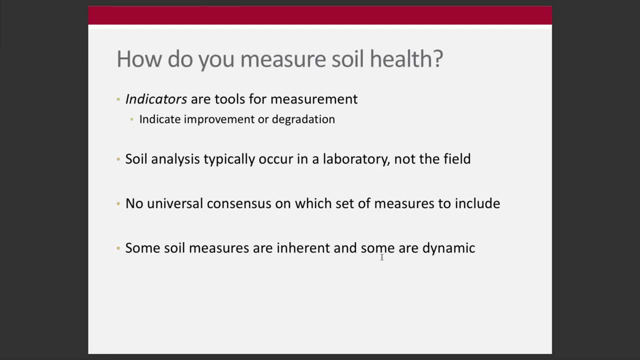 That's. you know that's a fundamental concept or a tenet of science. So there are many, many potential indicators, But there's some nuance or complexity in this. So indicators are a tool for measurement. It indicates an improvement or a degradation. 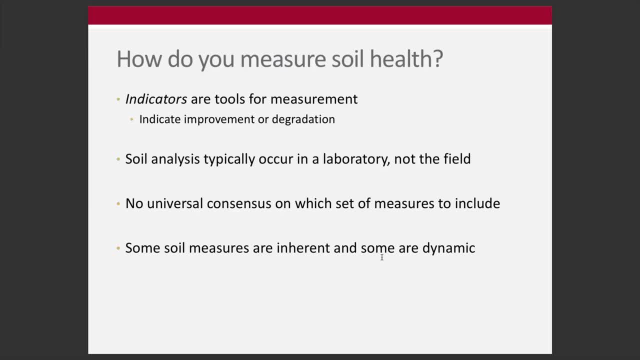 or just where you are Like. are you, you know, in a good range or a bad range? So soil analysis typically occurs in the laboratory and not in the field. That's another piece right Today, you know, standing here and not for the foreseeable. 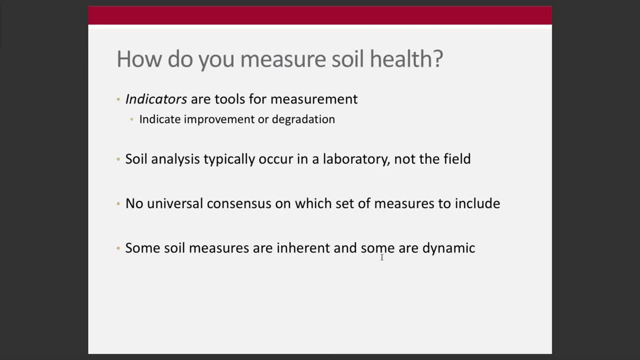 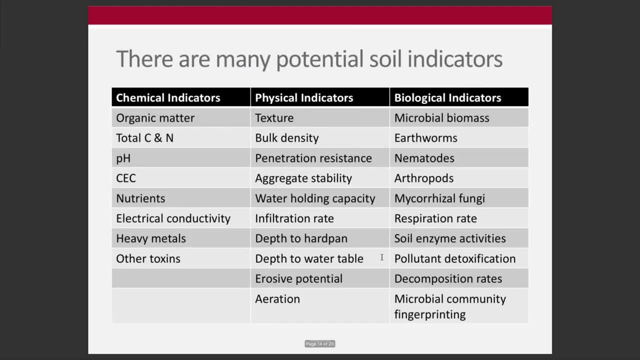 future will there be a universal consensus on what set of measurements to include. So this is a challenge when we actually try to pick which ones from these lists. you know We could go out and we can measure all these things on a soil. 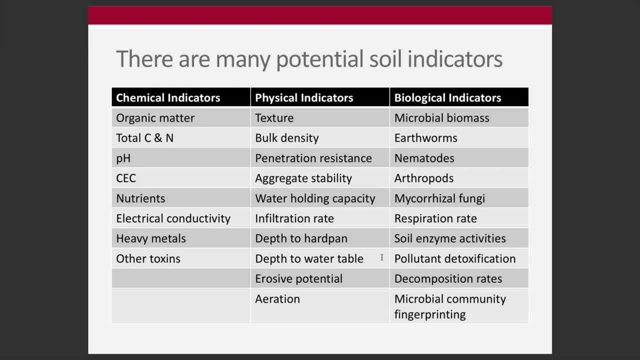 That's possible, We can do that, But it might take, you know, several weeks and it might cost you know, several hundred or even thousands of dollars to do that. That's not particularly practical. We need to pick ones that are very meaningful in each one. 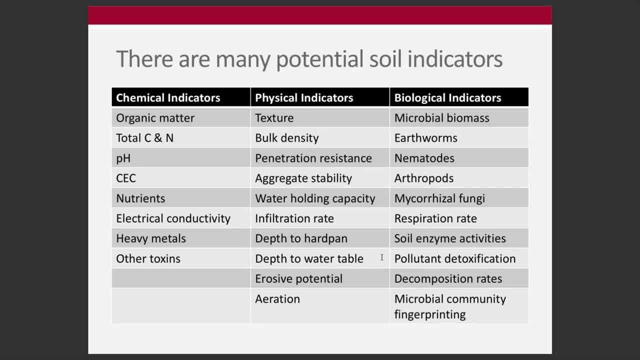 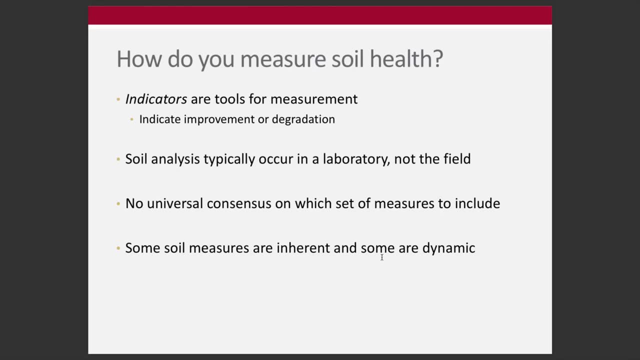 of these lists and help, you know, find indicators that reflect really important functions in soil and are not redundant with one another, okay, So another piece of this is: some soil measurements are inherent and some are dynamic. okay, So let's talk a little bit about that. 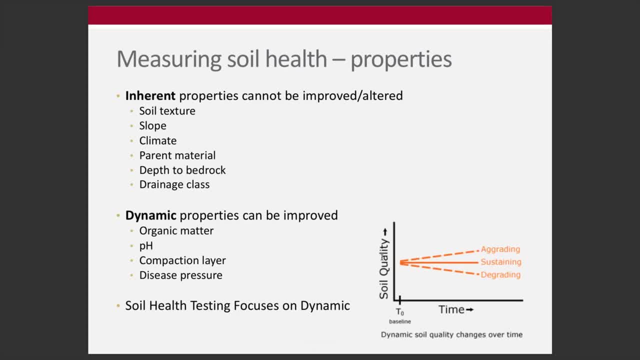 And this is an important thing- when we're talking about soils and we need to ground, like what soil health is and what it can do for you And you know, if we strive for soil health da-da-da, Like we are. so what does this mean? 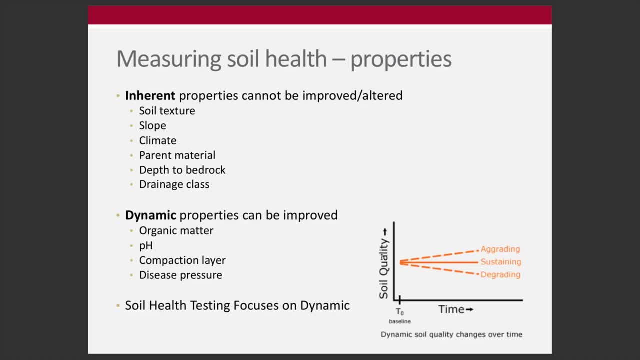 So we have inherent properties and dynamic properties. Inherent properties are like the genes of a soil right. They're properties that cannot be improved or altered. Things like the texture, the slope, the climate with that soil is in what it's developed. 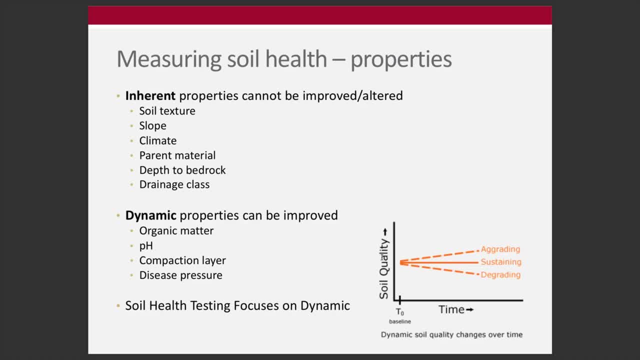 the parent material, you know, the feedstock of that soil, the depth of bedrock, drainage cuts- These are things that, no matter what we do, we're basically stuck with, right. So what we focus on in soil health? 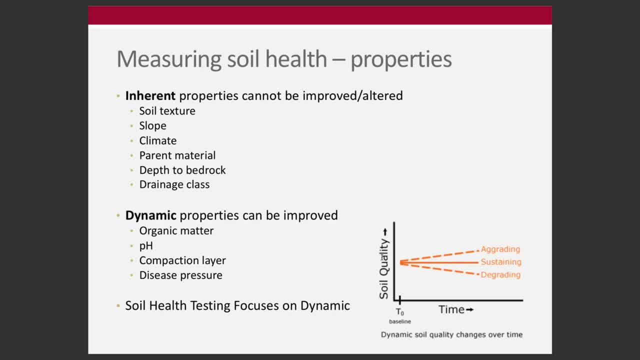 is these dynamic properties, These are things that can be improved with management, Things like organic matter percentage, the pH, the compaction layer, disease pressure, all these things that we can manage for. So it's just important to understand that we are never, ever, ever, going to take a say. 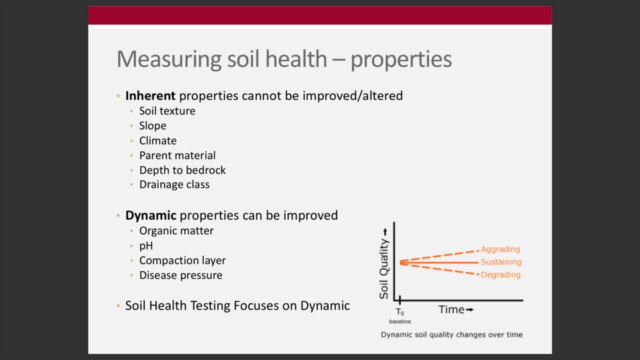 Hoytville clay in western northwest Ohio and transform that soil into a mollusk soil that we find in Iowa. okay, And we're not gonna take a sandy soil from Erie County and turn that into, you know, a really deep soil. 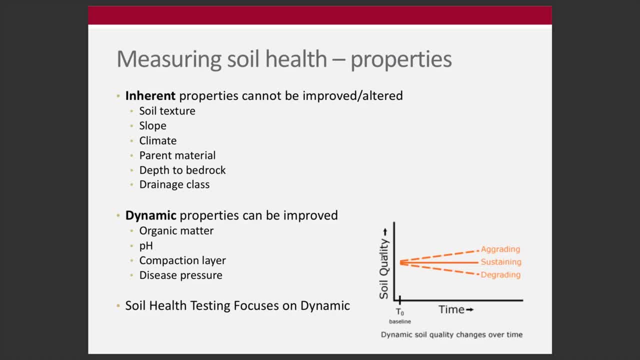 So we just have to understand that there's only so much that we can do with the soil in terms of, you know, altering its function and its production capacity. So we, you know, soil texture changes very slowly over time, unless there's some big erosive event or something like that. 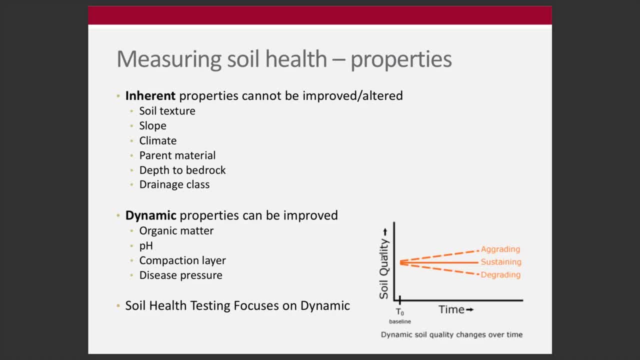 But you know, barring like major, major disturbance events, we're not gonna- you know we're not gonna- take a sandy soil and make it into a silt loam soil. It's just not gonna happen. So we have to like be. 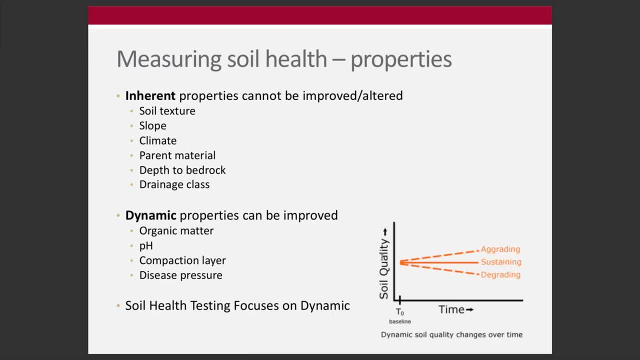 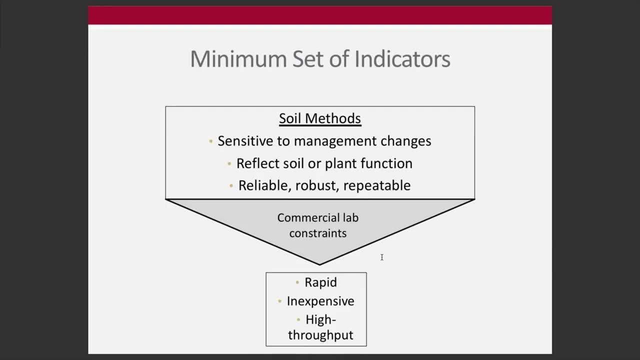 we have to be realistic and grounded in what we actually can do with the soil. okay, We have to work within our constraints, I suppose. So think of all this. you know that table that I just showed a few slides back with all these different measurements. 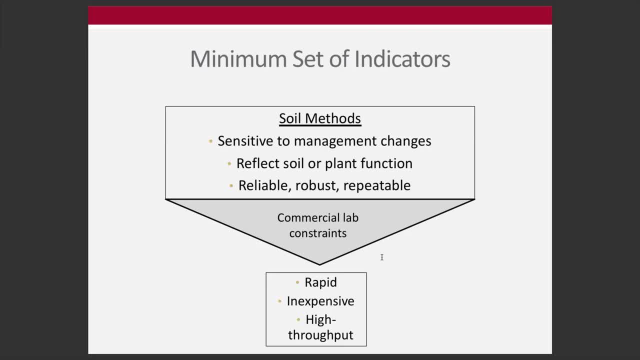 or indicators in there. So how do we do this? Well, how do we actually pick what a minimum set of indicators are so we can actually go through and measure and maybe quantify the health of the soil? So we are looking for indicators or measurements. 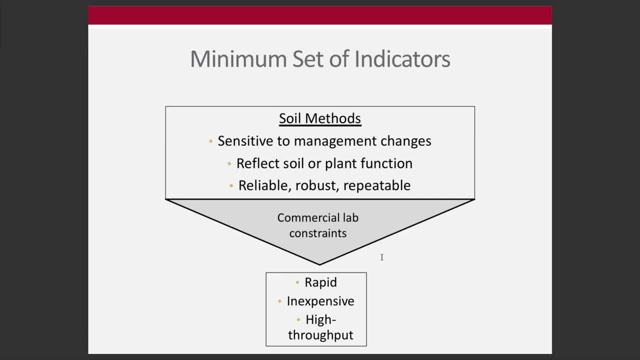 that are sensitive to management changes. We are looking for ones that reflect some soil or plant function. right to make it intuitive about what that is, We're looking for something you know, a measurement that is reliable, robust, repeatable. 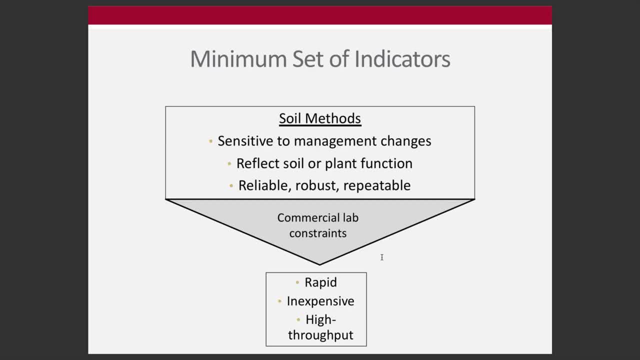 Something that's not gonna. you know that you get a value of 100 one day in the lab. the next day you go back and measure it again and you get a value of 250.. Like that's not helping. you know, us understand or repeat. 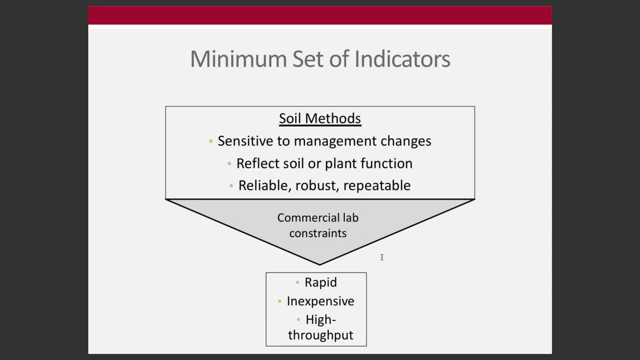 It's just, it makes that measurement a lot less reliable, And we'd like to kind of pull these together so that we might be able to be selecting from different functions or different plant properties or soil properties. okay, So then there's like: so we might winnow down a list. 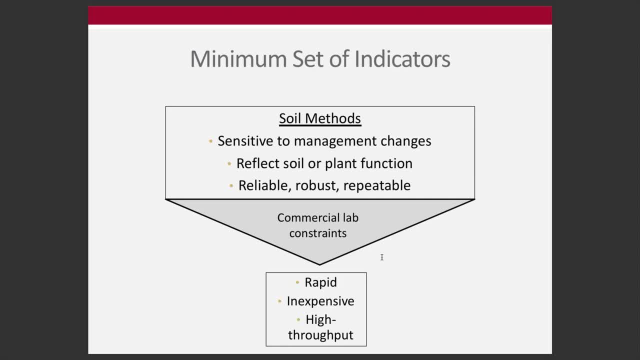 of indicators after we do, you know, say, look at these three things, or maybe four things, And then we just have this very kind of draconian winnowing again that happens, which is thinking about most of these measurements, Or at least this is kind of how I think about it. 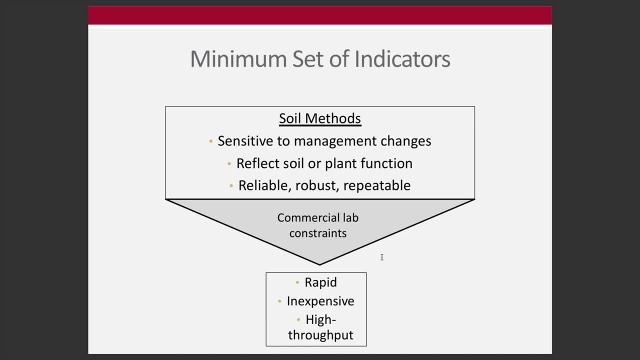 and what we spend quite a bit of time in my lab thinking about. We want soil health testing to be something that farmers do consistently right. That's. the ultimate goal is provide us an additional set of tests and information to help farmers manage soils. 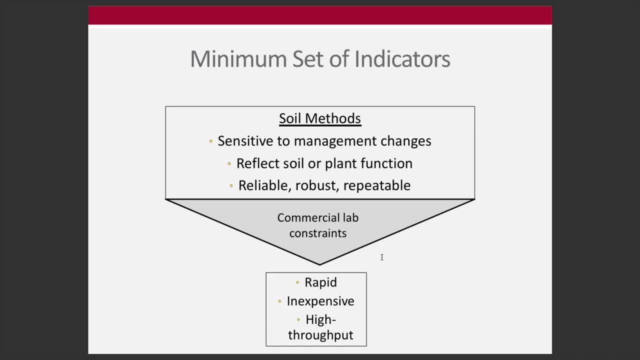 manage crops better. That soil is gonna not happen in a Ohio State. you know University, you know state, you know state, you know University lab. It's gonna happen in commercial soil testing labs. And so commercial soil testing labs have you know. 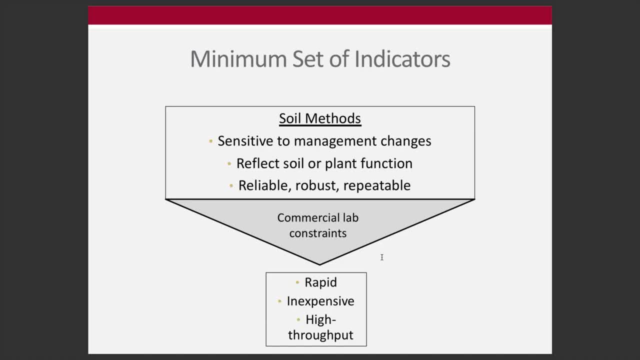 have constraints And those we could get into this a little more, but essentially those indicators have to be rapid. In other words, it can't take, you know, three or four weeks to get data back. It's gotta be something that you can look at and measure. 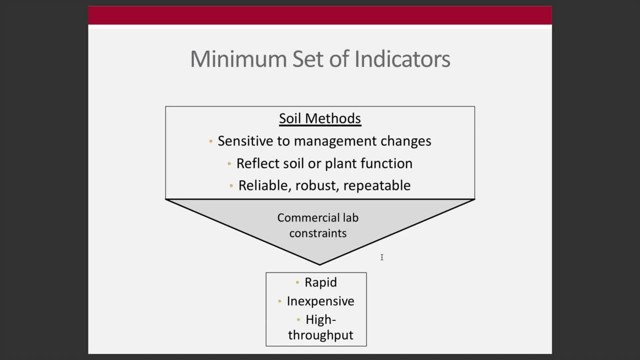 and get data back the next day or the next few days. It's gotta be relatively inexpensive, because farmers just won't pay several hundred dollars for a test. They're not gonna do it. It's just like part of the psychology And it's gotta be high throughput. 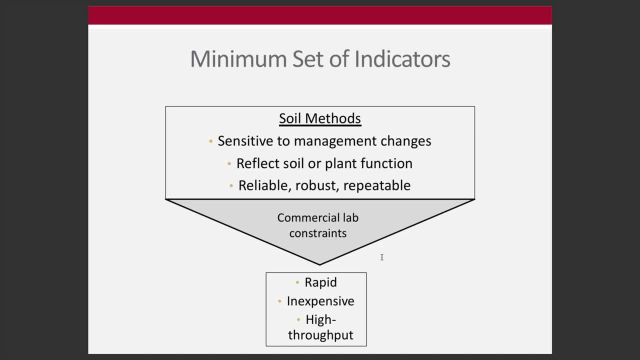 meaning you have to have the capacity to run several hundred, several thousand of these tests in a day. If it's something like that, you know you can only do 10 at a time. You know, I've got this machine and it only runs 10,. 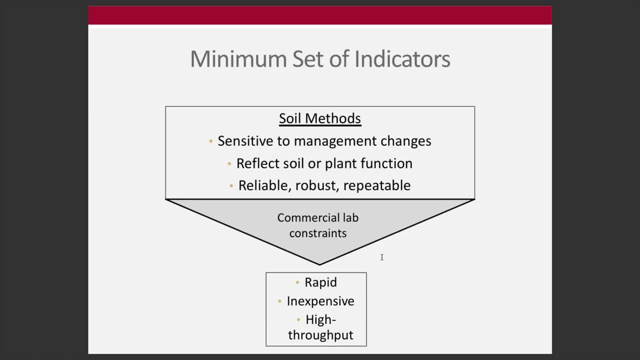 uh, samples a day. Well, you know, these are commercial soil testing labs. Our use, our laboratories that can process, you know, hundreds or thousands of samples a day- the big ones do- And so we have to have you know methodology or indicators. 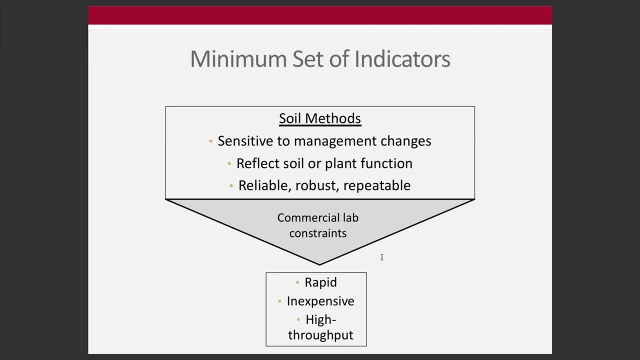 that will accommodate that, that will be able to handle, you know, that sort of throughput through their labs. Otherwise they're just not gonna pick them up, They're not gonna offer those tests And it's, you know, gonna be kind of a similar situation. 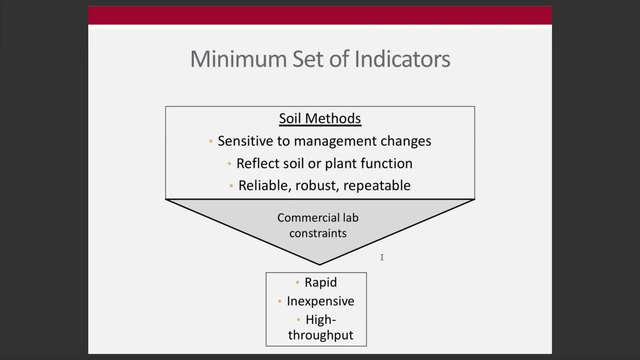 where we are, where the majority of commercial soil testing labs that do chemical testing do not provide soil biological testing. okay, And it's because there's been obstacle. I mean, there's a lot of reasons for it, But the, the, the tests that are offered commercially all meet. 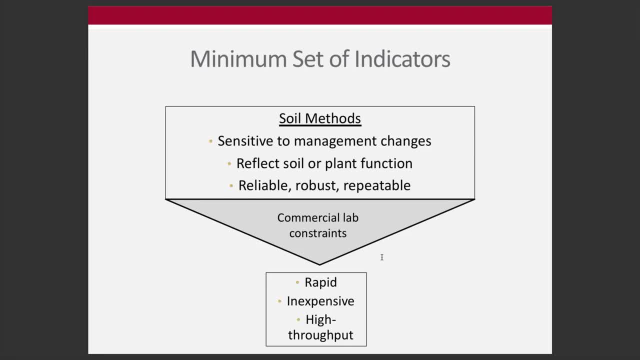 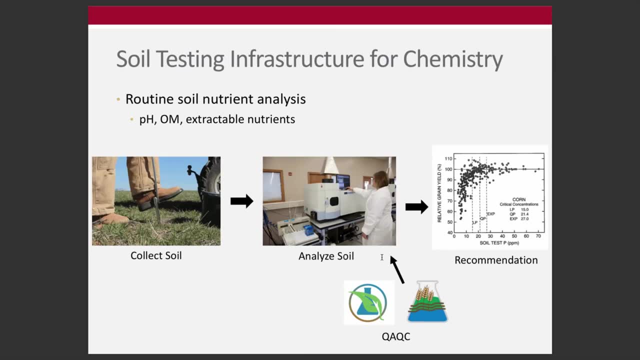 these criteria: They're rapid, they're inexpensive and you can do many samples in a day. Okay, Soil testing: we have a tremendous infrastructure in this country for soil testing right, And it's like easy to take this for granted. 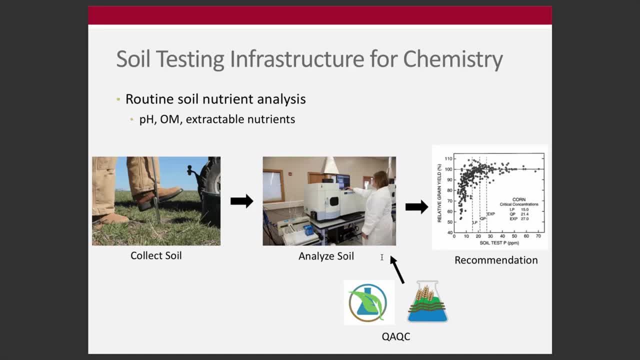 But anybody essentially can go out collect a soil sample. They can send it to a commercial lab and there's several to choose from. That lab has standardized methodology to analyze properties in that soil. There's been all this background work, you know. 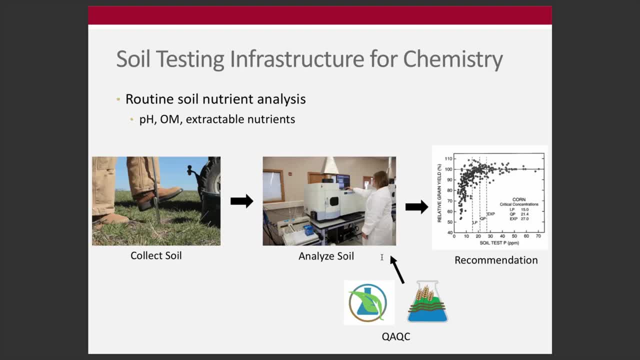 background work to develop recommendations for fertilizers, for example. This is, you know, we've talked about this already, And then there's all I've got this QAQC. but there's organizations, third-party evaluators or auditors that these labs commercial labs. 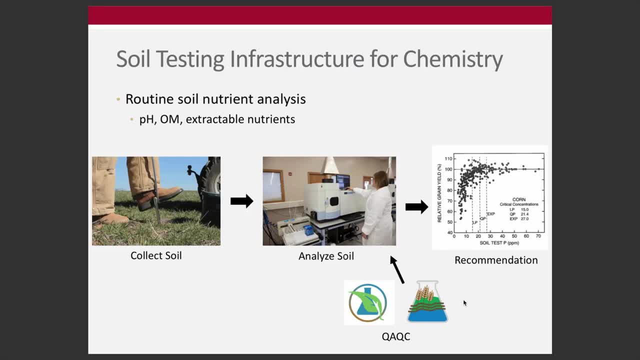 voluntarily subscribe to, And it's an accreditation of sorts to show that they are proficient And producing consistent values. And so you know, this is a whole infrastructure that already exists to give us things like organic matter, pH, extractable nutrients. 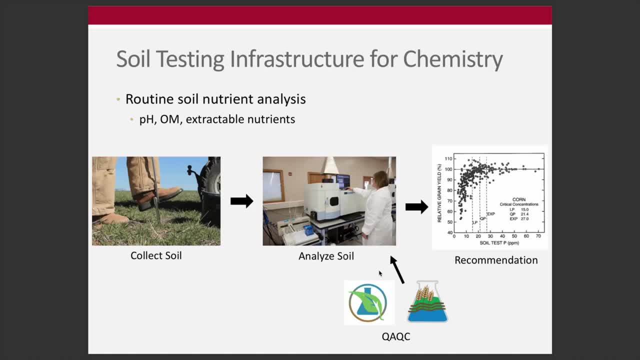 And then we can, you know, base nutrient recommendations on that right. So fertilizer recommendations are a direct result of soils that are collected and sent to commercial labs. So when we're talking about soil health, you know one of the things I mean. 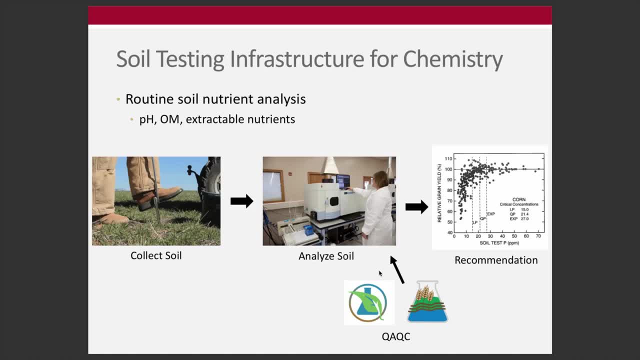 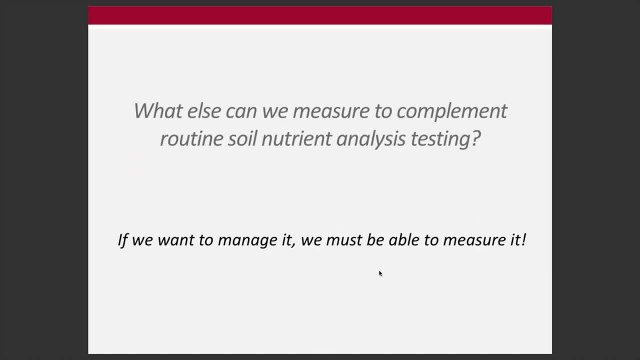 I come at it from a very applied perspective, I'll concede that. But you know, what we need to be able to do is we need to be able to not just measure chemistry, but we need to also be able to measure soil biology. 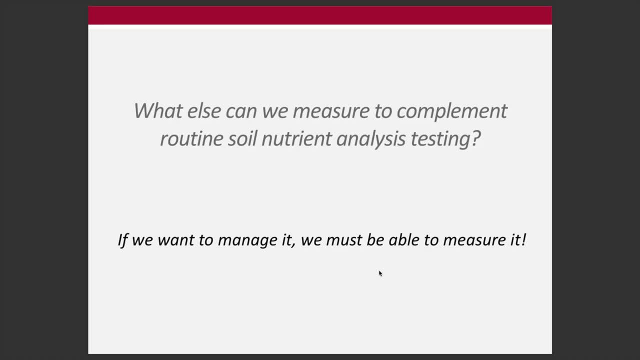 And we need at least have some kind of indicator of biology And we need to measure or have indicators related to soil physical structure, Because from a you know from a you know, from a you know from a soil conservation, soil management perspective. 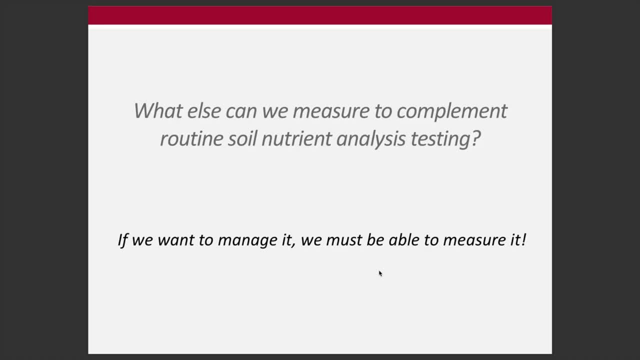 we need to manage the biology, the chemistry and the physical piece, you know, if we really want that soil to reach its full potential in terms of function. So and again, this is just about like developing measurements, indicators, a framework. 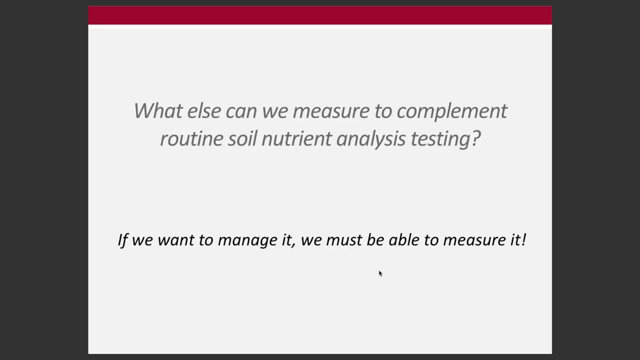 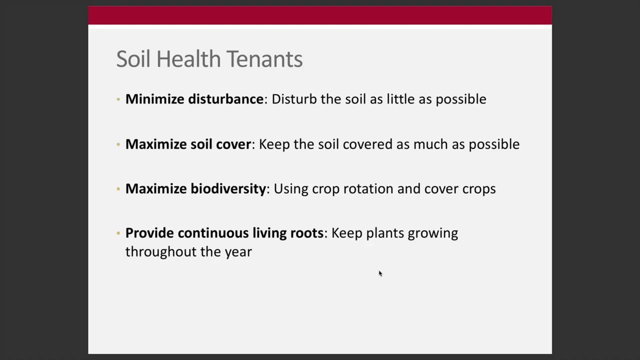 so we can measure things in addition to the routine soil nutrient analysis. So if we want to manage it, we've got to measure it right. I'll wrap up here just talking about soil health tenets, okay, So again, this is something that is, you know, very important. 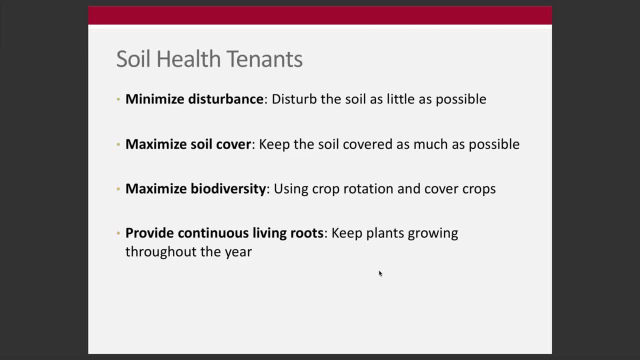 We need to- and this is kind of just capping off you know some of the soil health, But we just need to do the if we want healthy soil. this is all we need to do. This is all we need to do from a management perspective, right? 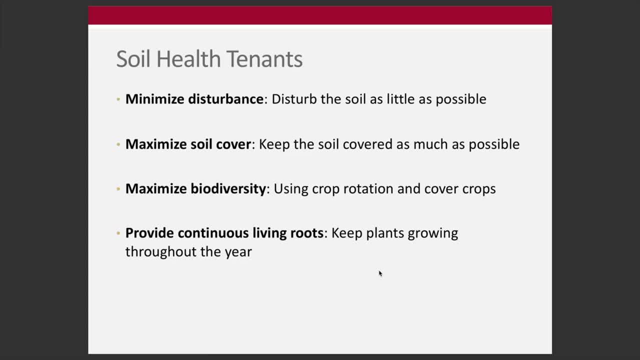 I mean, it's just so easy, but it's like the devil again is in the details. So we need to minimize disturbance. We know that when we are doing a lot of disruptive tillage or plowing our soil, health diminishes. 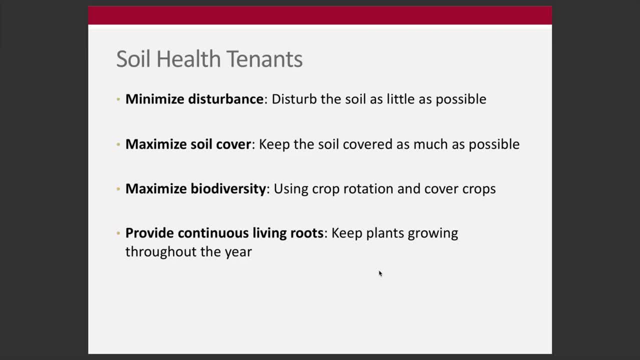 Our structure diminishes, The biology diminishes, et cetera, et cetera. We need to maximize soil cover, So keep the soil covered as much as possible. That means with live plant roots, okay, So keep residues on it. 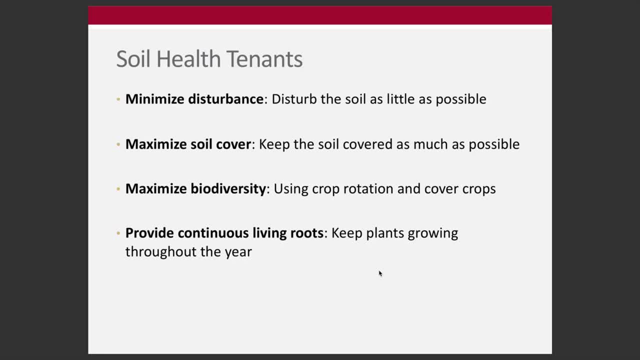 And keep, you know, wind and rain from hitting that soil and dislodging it and eroding it. We want to maximize biodiversity, So we want to. we know diversity serves lots of functions that we could talk about, But the more diverse plant species we have growing. 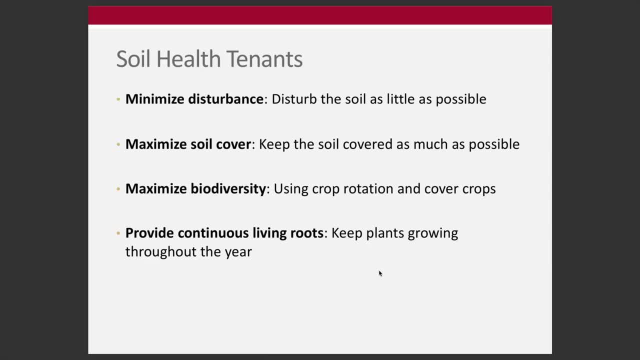 in a soil, the more different types of carbon chemistries that are being produced And you know we want to maximize biodiversity And the biological interactions with those plant roots and the decomposition process. So we just have complexity And with complexity of carbon substrate comes increased. 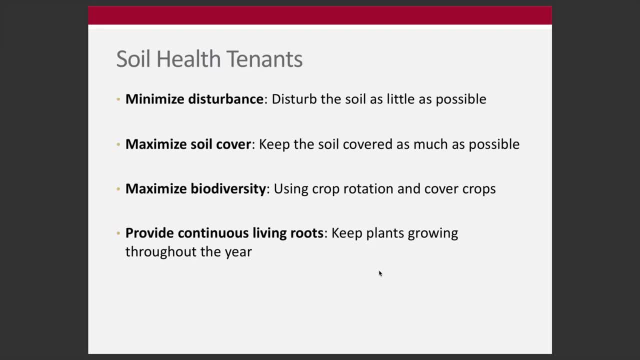 biodiversity or trophic structure, And with that means increased resilience, typically okay. So maximizing biodiversity? So just growing nothing but continuous soybean, year after year after year after year. Nothing else is not a way for us to get to a healthy soil. 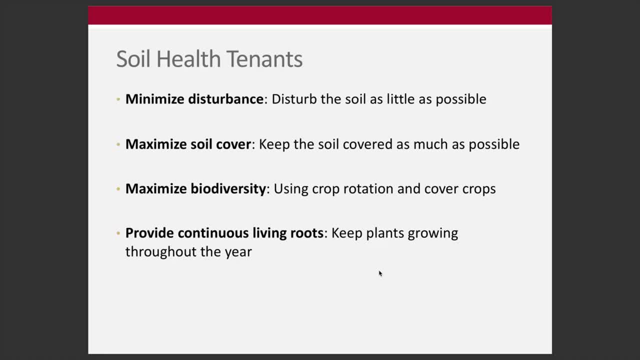 And then this last one is really important is providing continuous living roots. okay, So keeping, not just keeping the soil covered, but actually keeping plants growing throughout the year, to the extent we can. So this is important from an annual crop perspective, where you know some of our fields might be planted. 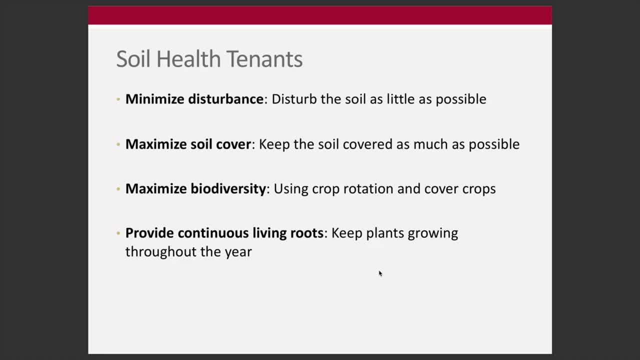 say in mid-May, early May, maybe not even until late May, And then basically, if it's, you know, corn or soybean or you know any sort of specialty crop that might be done, growing and harvested anywhere from, you know, late September to up to say, early November. 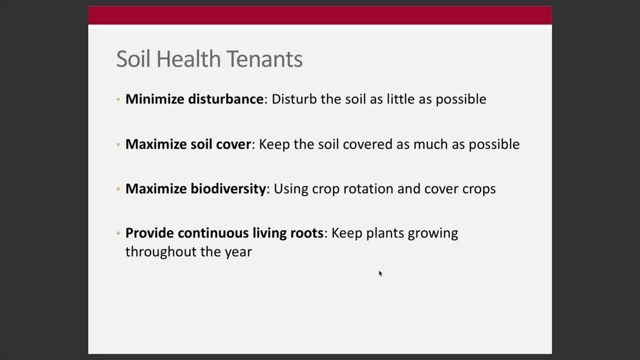 And even though that's the prime time, of course, for growing, there's still windows. There's a large window in the spring, say from March. you know maybe a couple of months from March to May, and then maybe a month and a half. 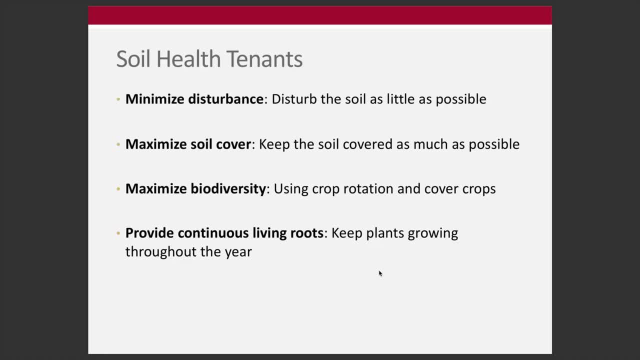 two months in the fall as well, where growth still happens Or there's, you know, above freezing temperatures or sunlight hitting the soil surface, And so in perennial systems or in systems that have cover crops with, you know, winter growth, for example. 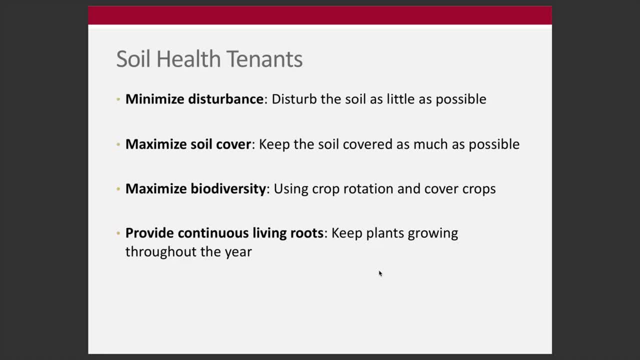 these are ways that we can provide continuous living roots, And we'll talk a little bit more about this. but roots are really important, of course, for lots of reasons, But, you know, providing that substrate, that feedstock for organic matter and feeding.